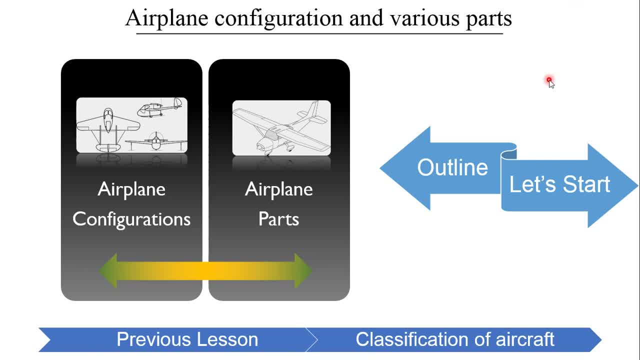 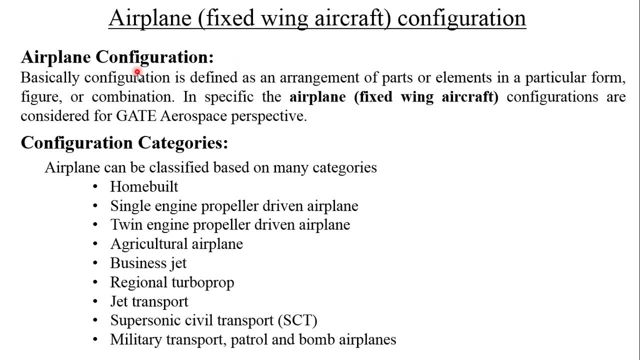 right top corner. that is this position. Let's start: What is airplane configuration? Before knowing about airplane configuration, we need to know what is an airplane and the difference between an airplane and an aircraft. Airplane is a subcategory of aircraft That is. 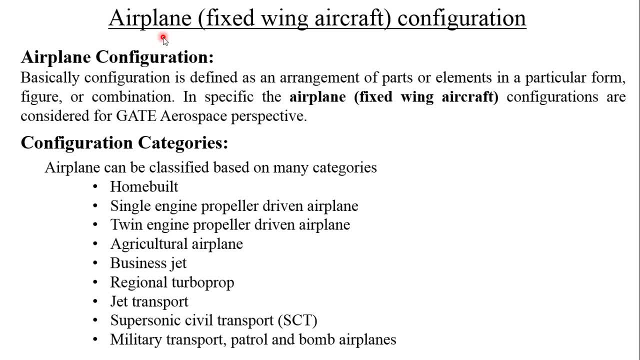 the fixed wing aircrafts are known as airplanes or aeroplanes. Configuration is nothing but a particular arrangement of parts or elements in a particular form, or figure or combination. This forms a particular configuration. In specific, the airplane configurations are considered for gate aerospace perspective. 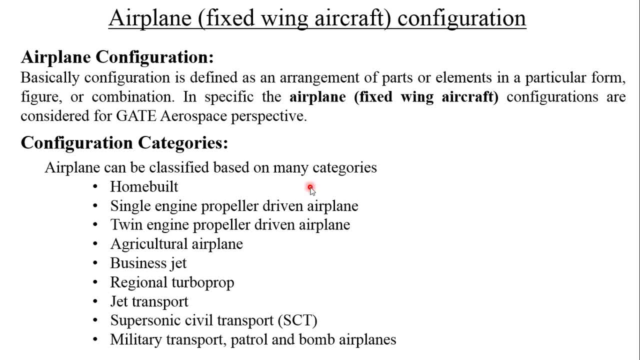 such that we need to know what is the configuration, because they will just name the configuration and ask a specific question about it. Here there are a list of nine different configurations of airplane, starting from home built to military transport. Each one has its own particular form of arrangement or a combination of parts. 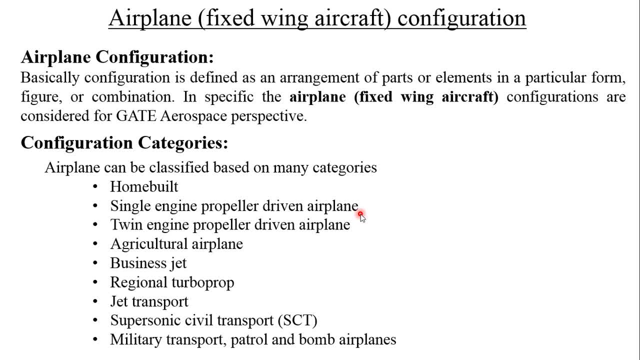 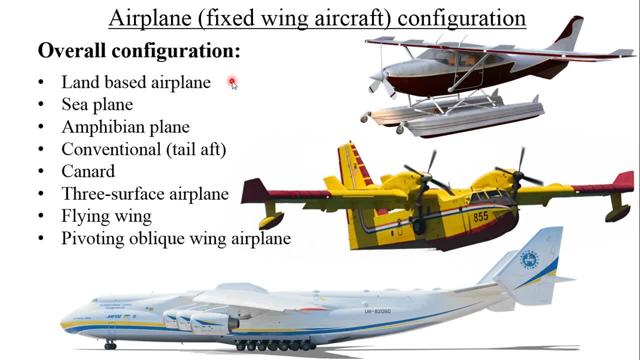 which is specific to that configuration. Let's see about them in specific. From an overall perspective, these are common configurations that can be seen around us Land-based airplane. Here is an example of Miria, that is ananten weakness aircraft, which is the largest aircraft of the worldziwa tener aircraft. 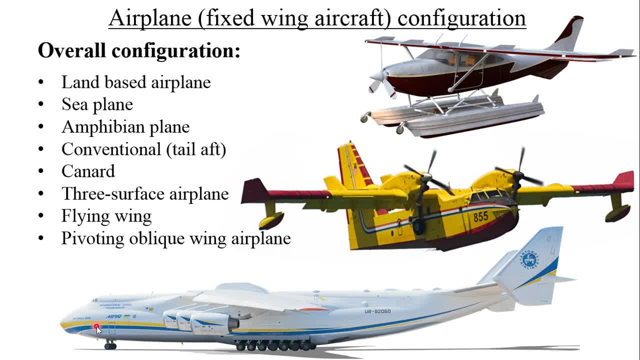 Let's see about them in specific: Earth plane Aircraft, incluso Aircraft Aircraft, which is the largest aircraft of the world aircraft, and this is a land-based airplane configuration. as we can see, the land-based airplane configuration has typical landing gears. that is retractable and the bottom portion isn't specifically designed for any purpose. 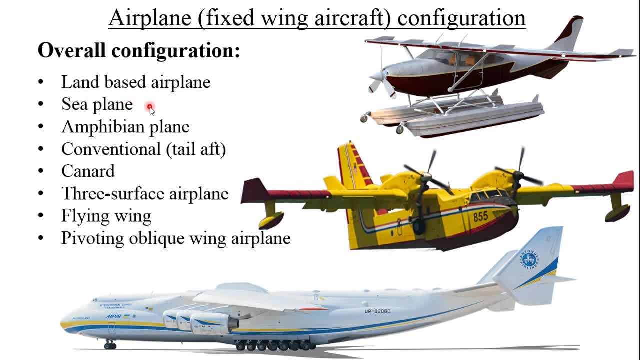 and it is common perspective. so the next configuration is seaplane. from the configuration perspective of seaplane here we can see that the bottom portion is replaced by a hull and we can see that the engines are mounted specifically above to avoid contact with water as seaplanes take off from. 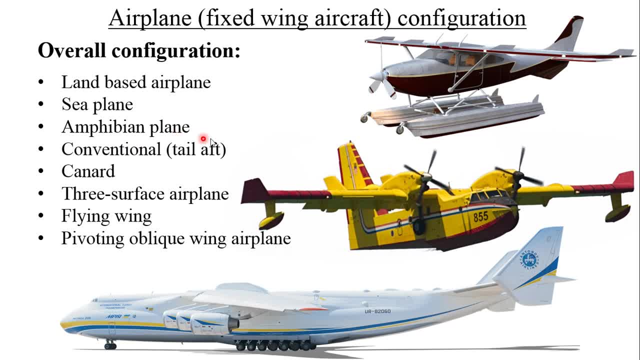 water bodies. amphibian plane. this is a combination of land and sea plane. here we can see that the bottom portion or the undercarriage is fitted with some kind of hull portion, that is, it can be able to take off from the bottom portion of the hull. 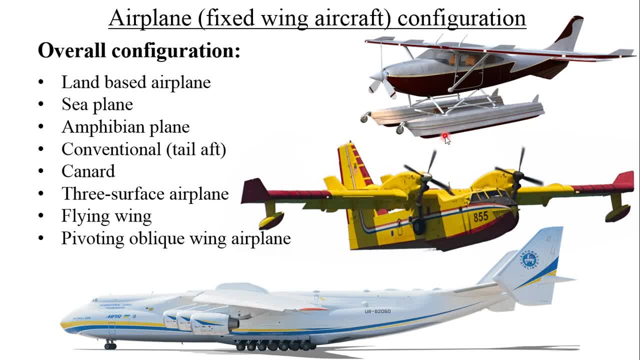 and it is also possible to take off from sea. for the purpose of taking off from land-based airports or landing strips or takeoff strips, the landing gear is kind of retractable version which is hidden inside the hull and it is dropped down for taking off and landing in. 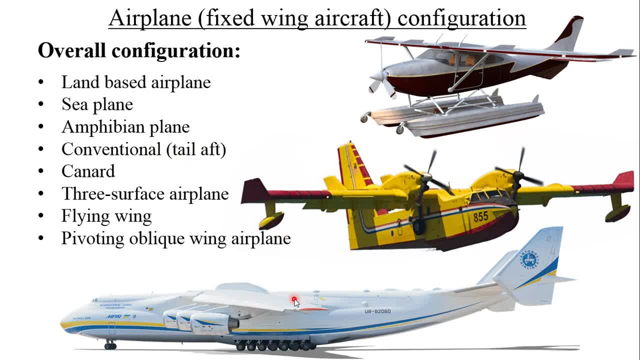 land-based landing strips. conventional aircraft is a typical aircraft configuration, that is, it has a tail after the landing landing strip is taken off from the landing strip and the landing strip is taken off from the landing strip after the wing, after the fuselage that is in the rear. 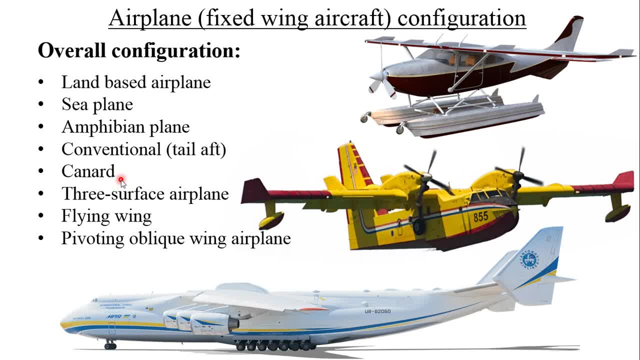 portion of the fuselage. canard configuration are common in fighter jets because it provides additional maneuverability for the aircraft. canards are nothing but the control surfaces which are attached in the forward portion of the fuselage in order to obtain additional maneuverability. three surface airplane in specific, we may not be knowing about. 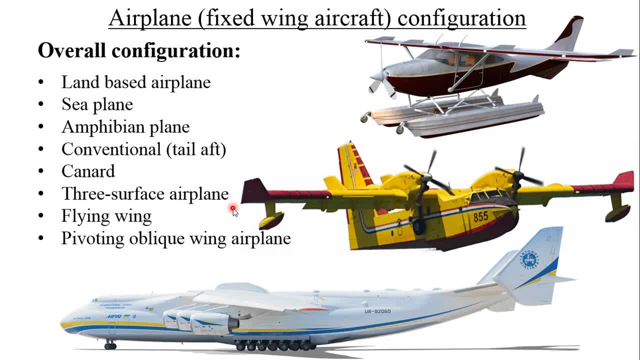 three surface airplane, but they are nothing but the airplanes with canard, a wing and a tail, that is horizontal tail surface. typically they will have three different surfaces or lateral surfaces for obtaining lift. first one is a canard, next the wing and then the horizontal tail or the stabilizer. flying wing aircraft or has 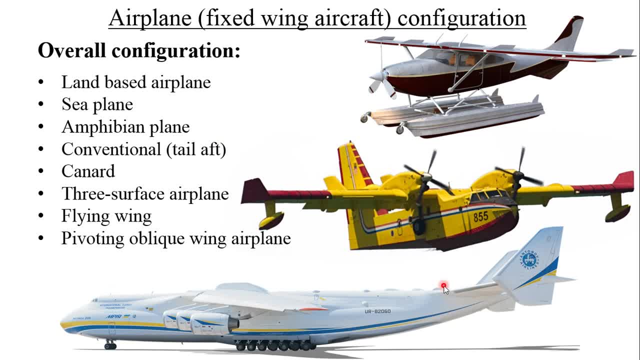 a typical triangular kind of body without tail, that is, the fuselage is integrated within the wing section. piloting oblique wing airplane. it is nothing but the airplane with a wing which isn't at a particular 90 degree angle or some particular angle. instead it is in some 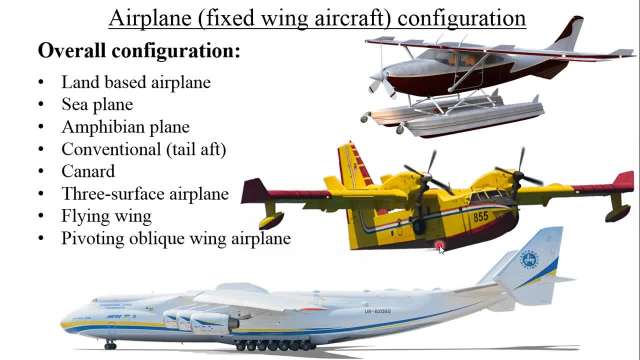 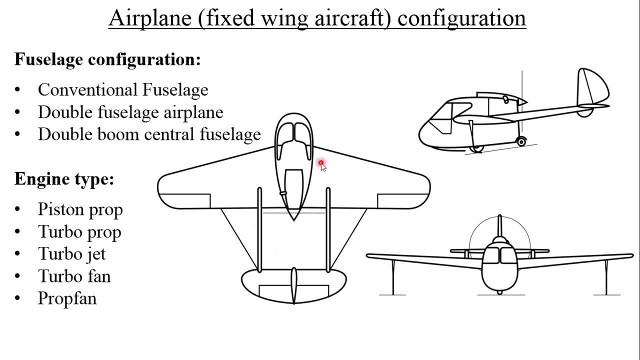 angled position, that is, it is placed in an oblique angle. so here is a typical example of a wing with a tail. it is a fuselage integrated within the wing section- typical example of flying car configuration- and it has twin boom and this is a particular. 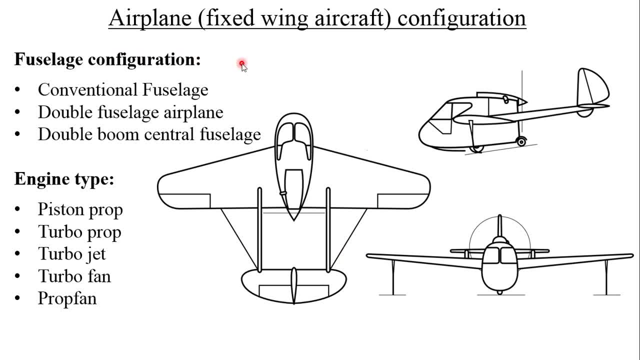 kind of configuration. so fuselage configuration, when we learn about the configurations from the fuselage perspective, that is, the configuration is based on the arrangement of fuselage or the design of fuselage. conventional fuselage is the typical fuselage which we see around in commercial airplanes such as a320 or Boeing 747, or most of the commercial airplanes, or 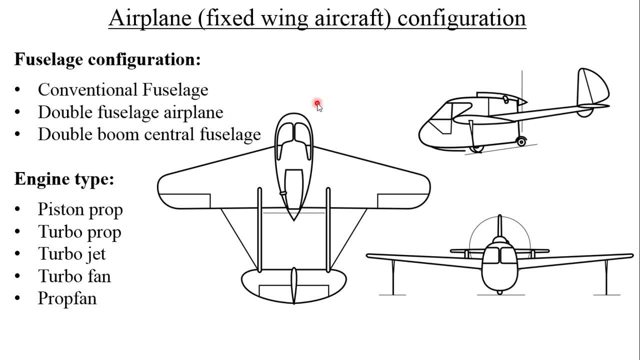 passenger crafts. double fuselage airplanes have two fuselage, that is, they have two areas where the passengers can be seated or the payload can be carried, and this is a rare configuration. and the next one is double boom central fuselage, and this is the typical example of a double boom central fuselage. we have the fuselage in the center and it 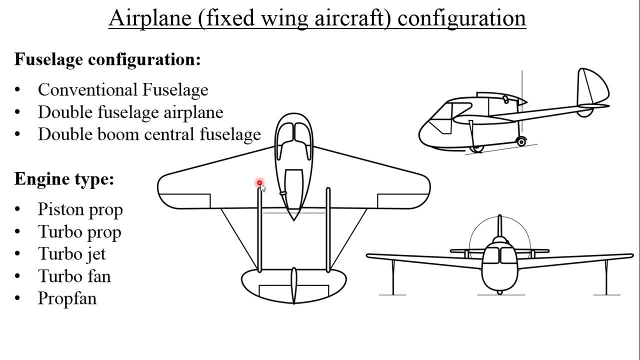 has twin boom. that is, boom is nothing but the tail to wing or fuselage attaching portion, that is. this is the boom structure. so double boom. it has twin boom structures. the configurations can also be based on engine type. it can be either piston, propeller engine, turbo engine. 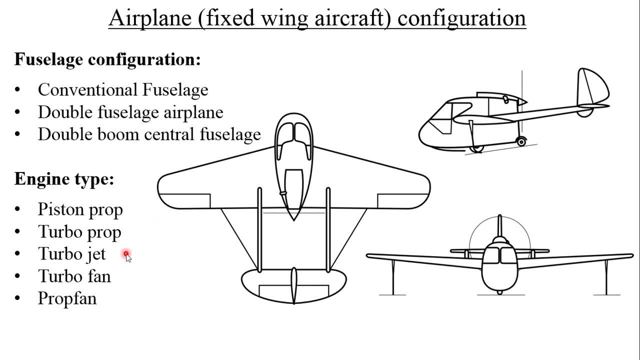 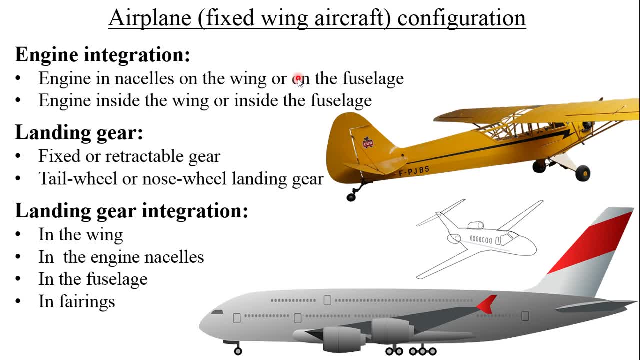 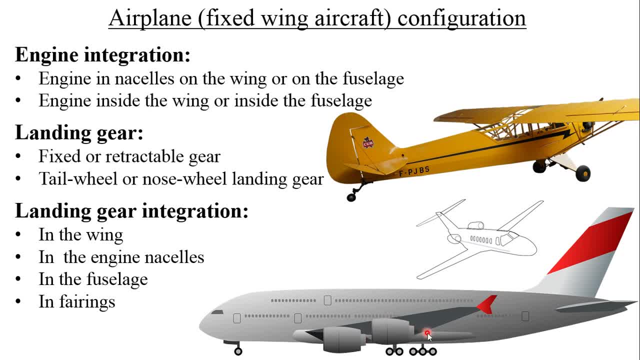 but these padded structures within which the engines are placed. so it can be either within the nasa, that is, under the wing, or on the wing. so here we can see it is an underwing and here we can see that the engine inside the wing or inside the fuselage, it is inside the fuselage, it is attached above the fuselage, over here. 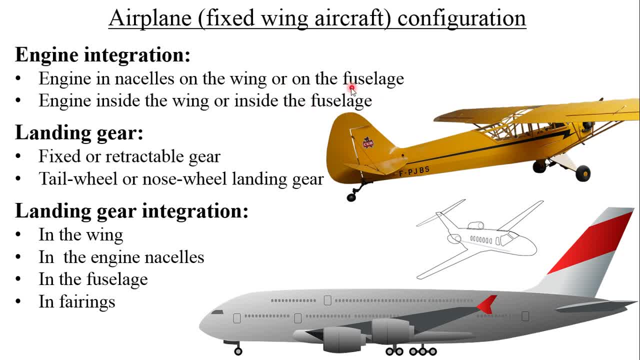 and in fighter jets we can see that it can be either attached inside the wing or inside the fuselage. inside the wing configuration is very rare but still there are prototypes and working models that are decommissioned model one of the fighter aircraft from british airways or 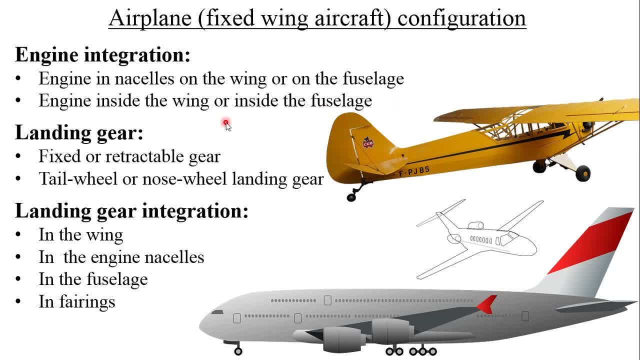 british air force was having a configuration of buried wing, that is, the engine was buried within the wing but it wasn't efficient so it was decommissioned. airplanes can also be configured based on the landing gear type, that is, either it is fixed or retractable landing gear. 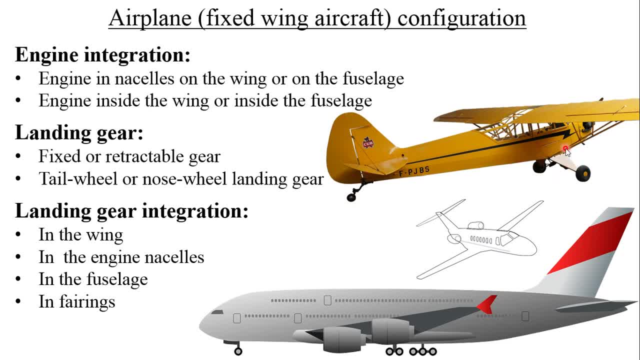 here. this is a typical example of fixed landing gear, and here we can see the landing gear can be retractable within the body. this is retracted in order to obtain lesser drag. the next configuration is tail wheel or nose wheel landing gear. the landing gear can be either placed in the print that is below the nose or 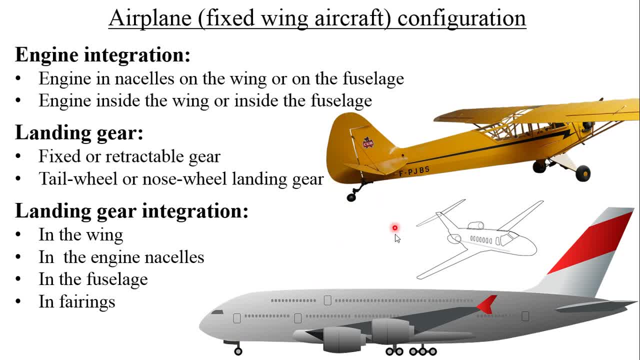 near the tail. so this is a tail dragger configuration and this is a nose wheel landing gear. it airplanes can also be configured based on the location of these landing gears. that is, either it is under the wing or inside the engine nacelles or in the fuselage. this is the example of inside. 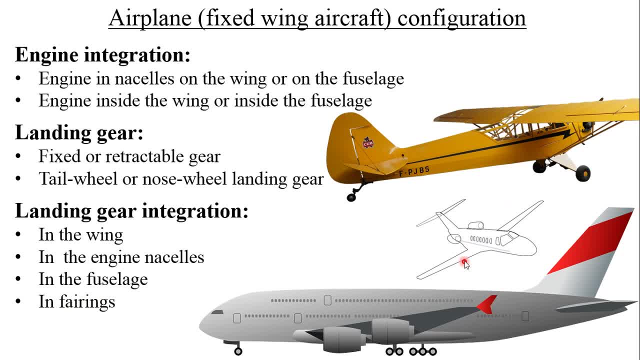 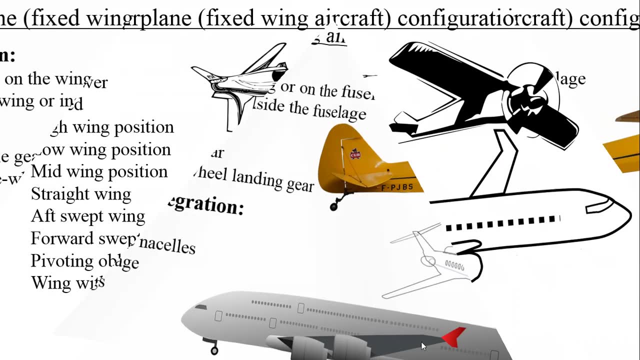 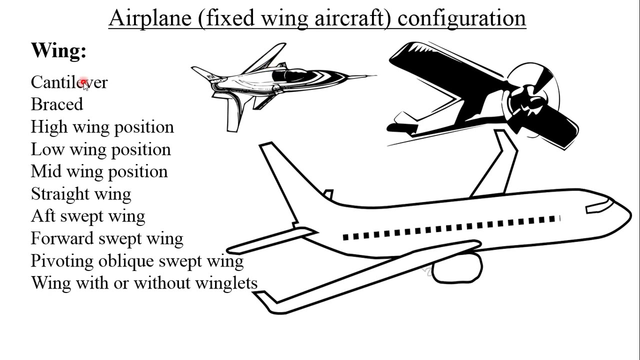 the fuselage or in fairings, that is, the landing gears are separately retracted or positioned within a fairing. so this is example of fairing, or sometimes it is attached below the fuselage. now, discussing about the airplanes configuration based on the type of wing, we can be seeing the following configurations: that is, it can. 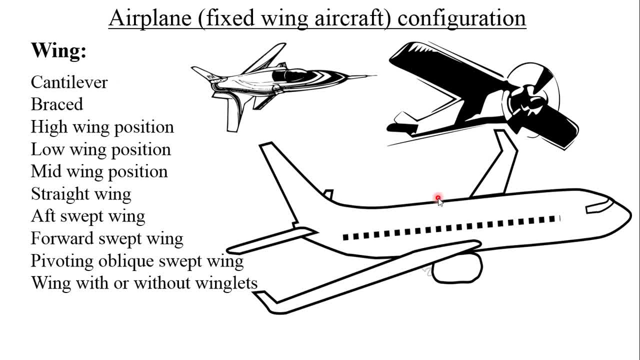 be either: cantilever. cantilever wing is nothing, but it is fixed at one point and it is free at the other. brace wing: the wing structure has a support from the fuselage, that is, you can say that the wing is supported by a brace. like this you could have seen in the 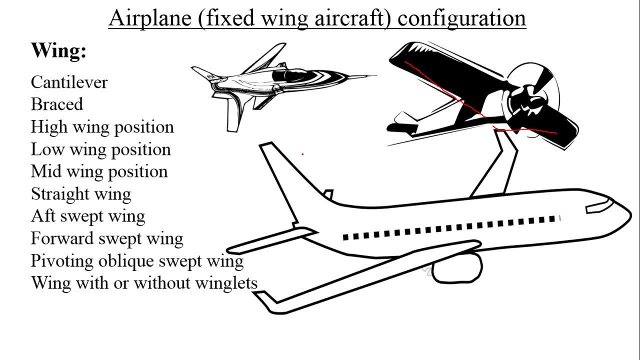 world war. i'll friends, but it is in common. now still cessna and other kind of two city aircrafts use this base wing concept. high wing is that the wing is positioned above the fuselage, low wing is where the wing is below the fuselage and the mid wing is where the wing passes through the fuselage. 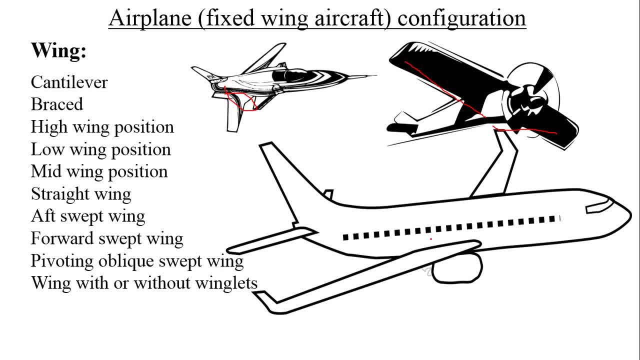 in the middle portion. straight wing is that the wing isn't swept back. so this is an example of swept back and this is the example of swept forward. and here we can see the wing is straight. so after swap, wing is nothing, but the wing is swept- uh, in the backward direction. 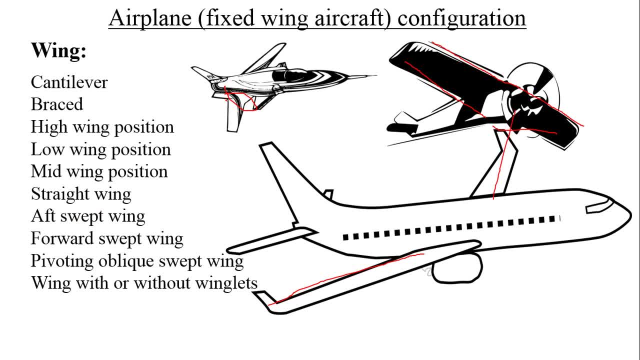 if we back angle is provided, forward sweep is that the wing is swept by uh forward in the reverse to the swept back configuration. pivoting oblique wing is nothing, but the wing isn't placed in a straight manner. instead, the wing is placed in some oblique angle. it is very rare configuration. 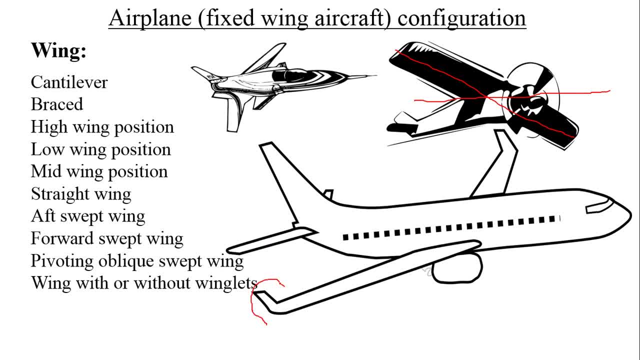 and wing width, or without in winglets. so these are known as wing lights and these are used to reduce the induced drag of an aircraft. so here we can see the aircraft is with winglets and here these two airplanes are typical examples of aircraft without winglets. 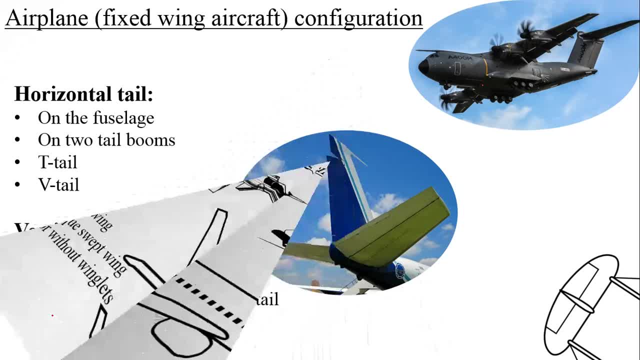 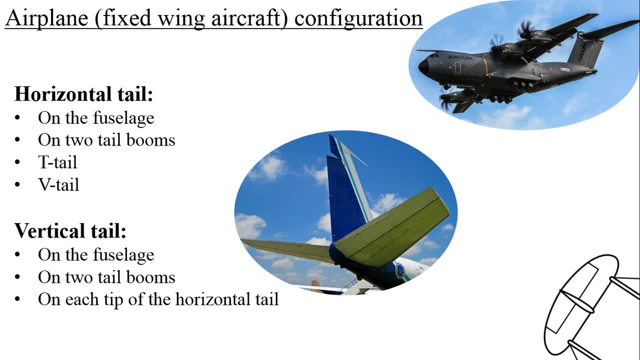 so i'm discussing about the airplane's configuration based on the horizontal tail arrangement. so this is the horizontal tail portion and the opposite is the vertical tail portion. so either the horizontal tail is placed on the fuselage- here we can see: this is the fuselage and the horizontal tail is placed. 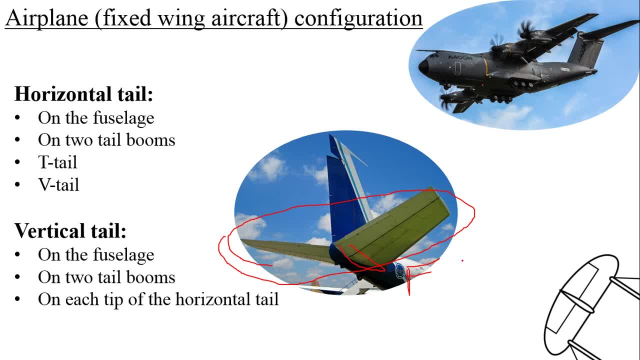 on the fuselage or on twin boom, twin tail booms, or- this is a typical example of the horizontal tail being placed on twin booms, boom number one and boom number two- and either it is having a detail configuration, so the tail, the horizontal stabilizer, is placed above the vertical tail. it will have a t-tail configuration. 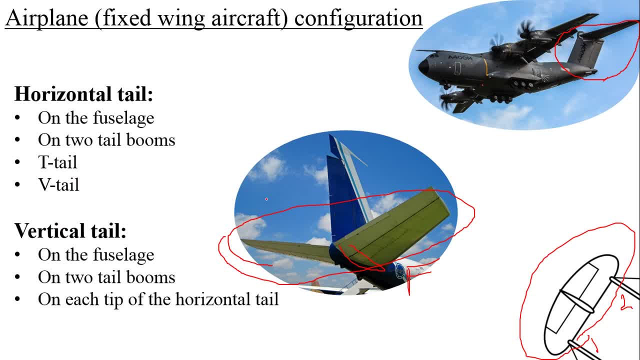 similar to this and v-tail configuration is common in fighter jets. that is the tail. horizontal tail is placed in kind of v-shaped structure, so vertical tile. this is the common example of vertical tail and it is the horizontal portion of the tail which is responsible for the yawing. 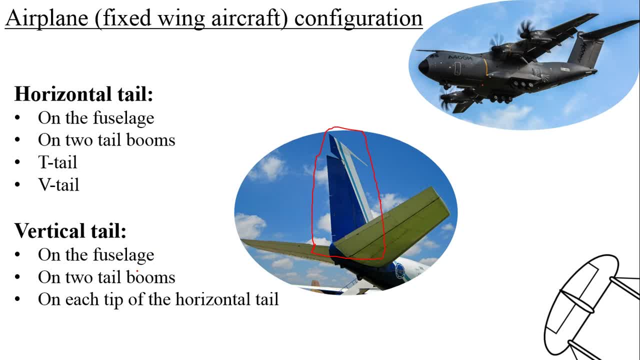 motion and the first configuration is on the fuselage. so here we see the fuselage, and the tail is placed on the fuselage or on the twin tail booms. so here, if the tail was placed in similar manner like this, on the two booms, boom number one and boom number two, it would be an 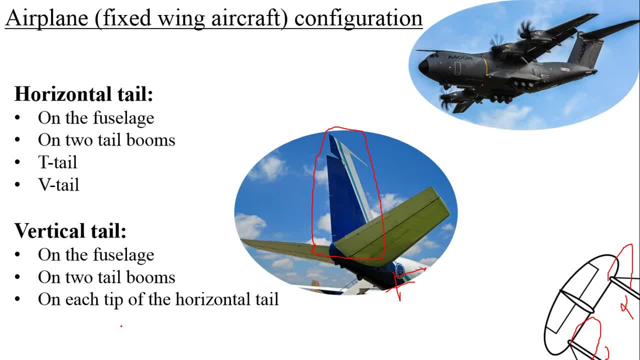 twin tail, vertical tail configuration on each tip of the horizontal tail. so in antenna media we did see that each horizon, that is, there was a horizontal tail and the vertical tail was positioned on the tips, that is, each tip of the horizontal tail, that is, it will be forming. 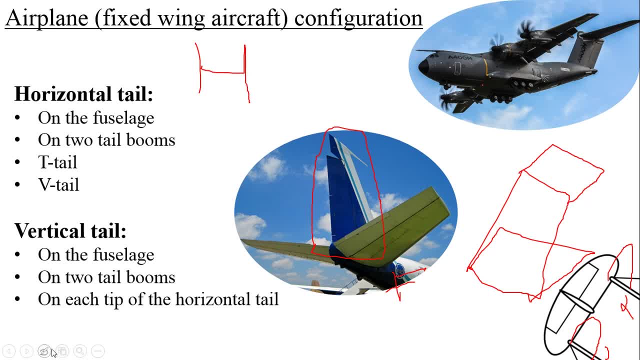 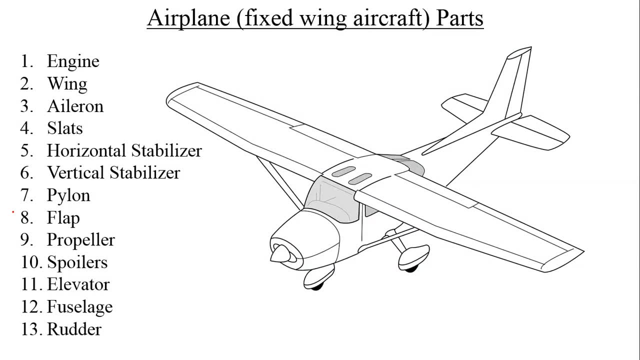 kind of h configuration of tail. now moving on to the next portion of the concept, the airplane part. as i said, airplane will be having the fixed wing and uh parts of it. there are typically 40 lakhs parts in an airplane that is a commercial passenger craft. but specifically we need to know: 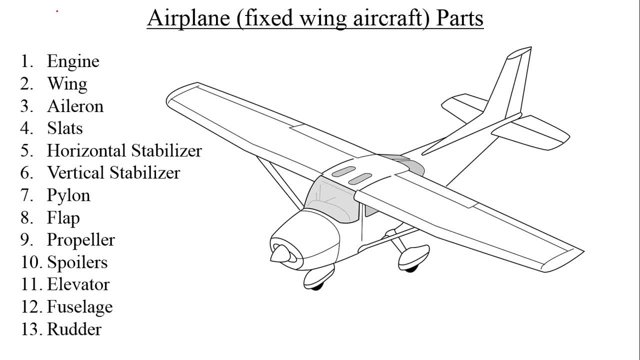 about these following 13 common parts, so they will be having subsystems and other systems supporting these parts which uh counts on for to that amount. these 13 are the main parts and we need to be able to identify it on any kind of airplane. so engine from the perspective of this aircraft, the engine. 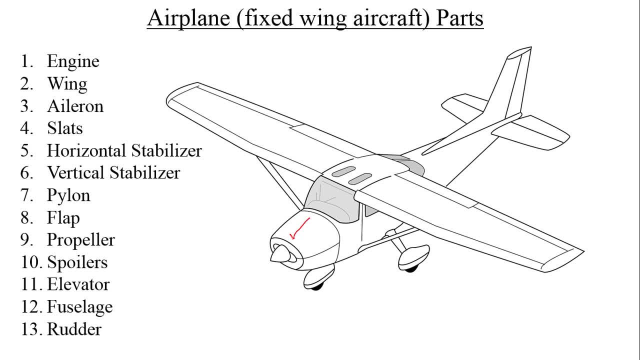 is placed in the forward portion of the aircraft and this is where the engine would be placed and here the rotor is connected and we will be having a propeller over here which will be helping the aircraft to thrust forward wing. so this is the wing from here to here, and this is 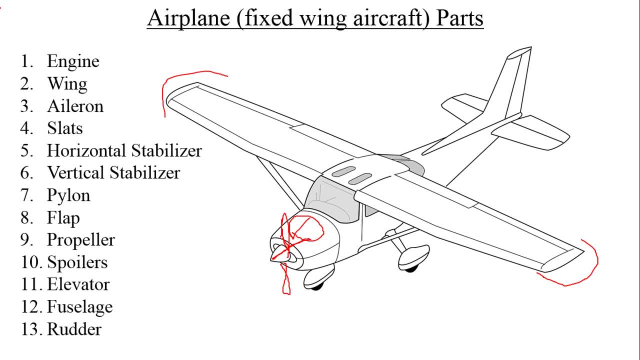 a major lift providing device of that airplane: aileron. ailerons are used to provide roll and ailerons are placed on the either tips of the wing as it provides the rolling motion of the aircraft: slats- this aircraft doesn't have slat specifically, but slides are the devices which are 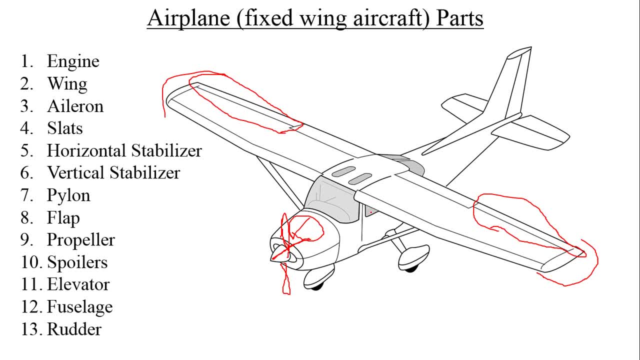 placed on the wing and it can be either leading edge slats or trailing edge slats and horizontal stabilizer. so this portion is specifically known as the horizontal stabilizer and uh, it cannot be controlled, but it is a stable device or a part, thus the name stabilizer- horizontal stabilizer. 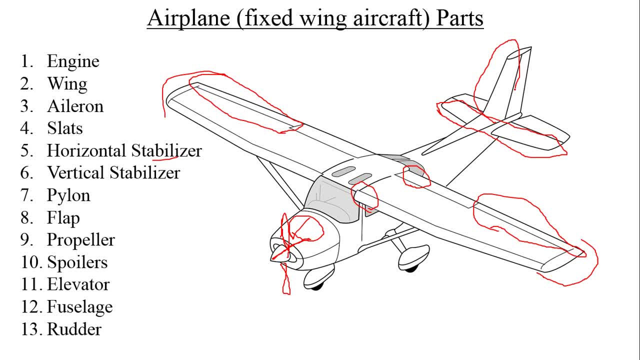 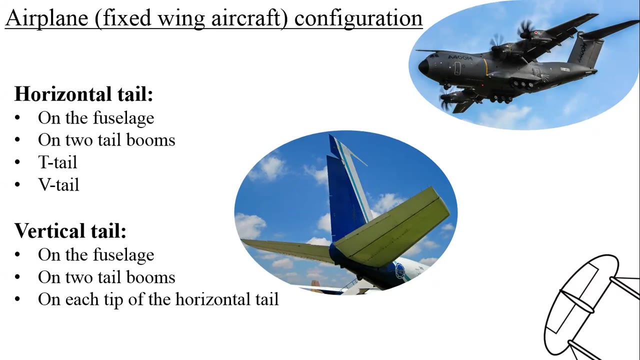 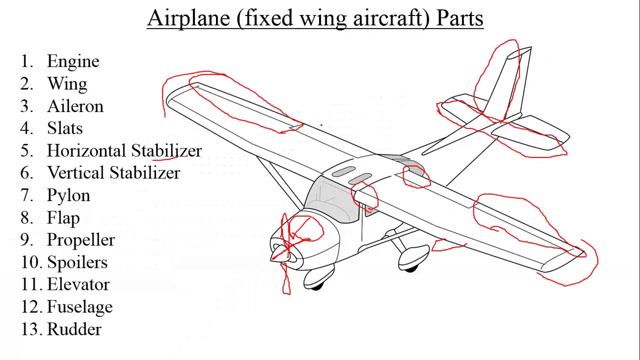 vertical stabilizer. this portion is known as a vertical stabilizer and next pylon. pylon is where a device or a part which is used to mount the engine we could have seen in aircrafts such as these. here the engine is mounted on the wing and the connecting unit is known as file, and next is a flap. flap is attached. 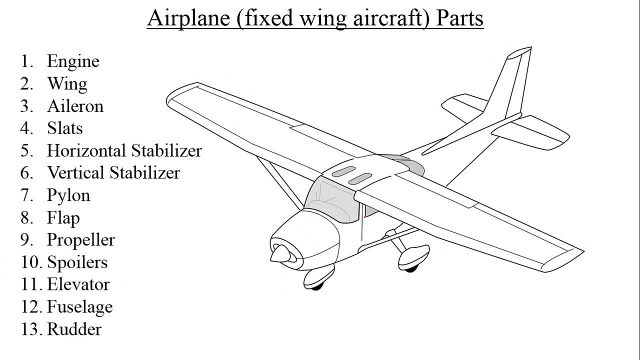 near to the fuselage. so here we can see that this is the flat region on either side of the wing, near the fissure L, and this is the sleeve and this is the front area and these are in front. here we can see that on either side of the wing, here the fuselage and thisор 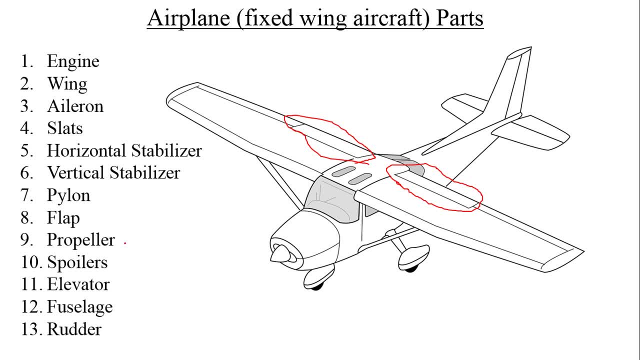 the. so here we can see that this is the flap region on either side of the wing. here Arga was continue on either side of the fuselage and thisor is a major lift providing device propeller. as i said, propeller is either attached in the forward. 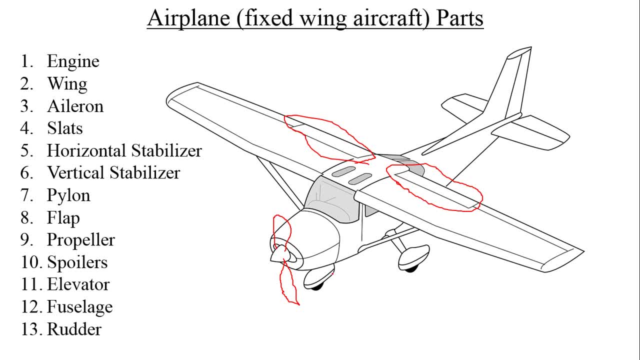 portion of the aircraft, and this is a tractor configuration, or there is puller configuration, or, if the propeller is attached behind the aircraft, it is a pusher configuration. so next one is the spoilers. spoilers are mounted on the wing surface and, as the name suggests, spoilers are used to spoil the lift or increase the drag for helping the aircraft to slow down. 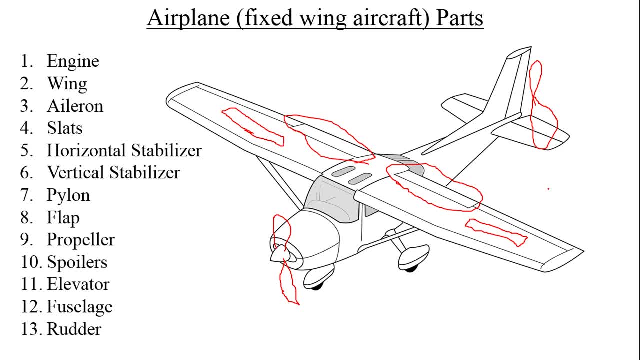 in cases of braking in fighter jets they are used to provide or achieve sudden turns elevators. elevators are attached behind the horizontal stabilizers of the aircraft and it is used to provide the pitch of the aircraft fuselage. so this portion where the payload or the passengers are seated are known as fuselage.